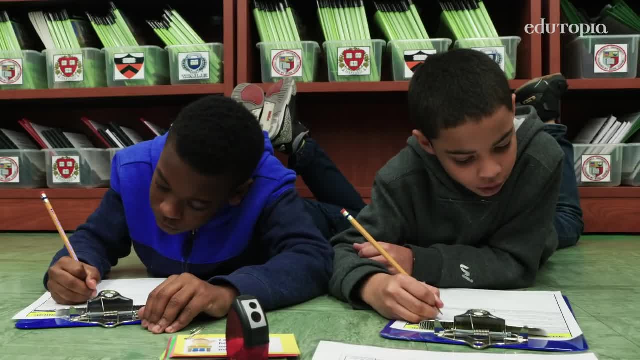 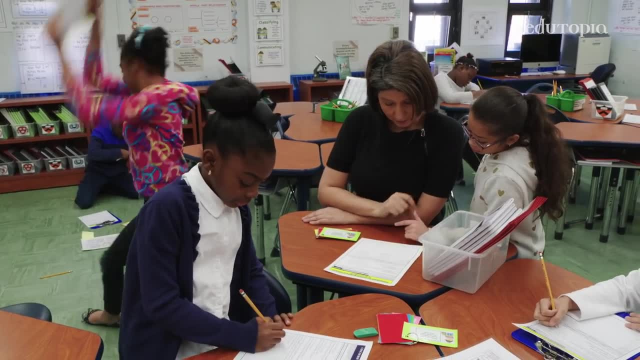 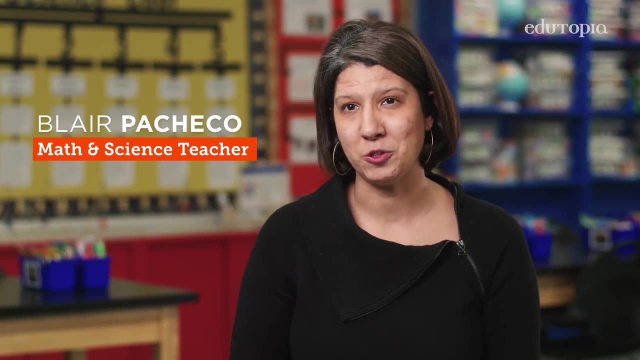 We use the procedure so it's easier to understand the problem and when you're looking at it you know what to do. It helps them to become more organized with their thoughts. It becomes almost like a checklist for them. It's also important because their reading skills are going to improve also throughout. 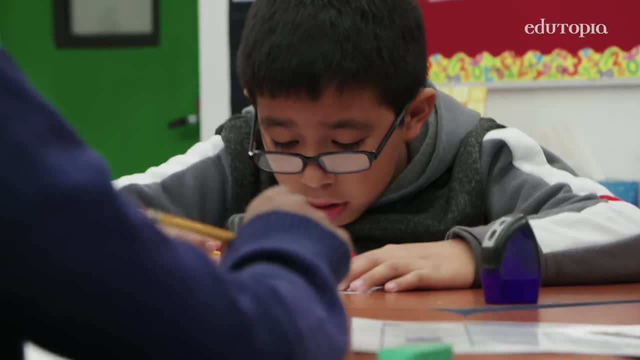 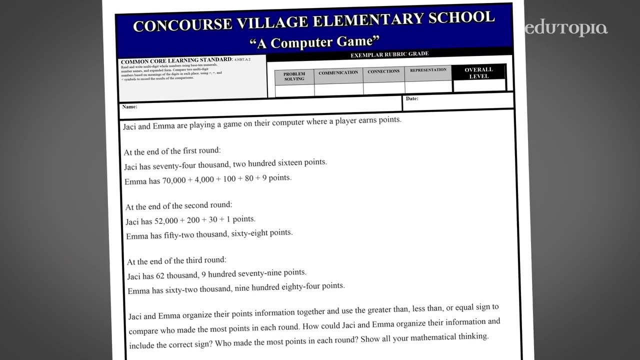 the whole entire time. They're really honing in on specific words, So it's going to help them get the gist and really understand the content of what they're reading. The math problem was about JC and Emma. They were playing this game on their computer and they were trying to see who got the most. 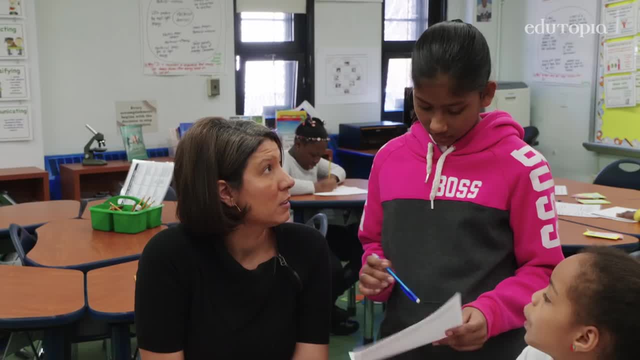 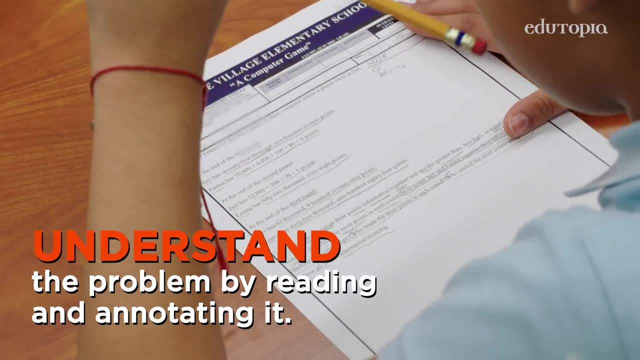 points. So who made the most points in each round? In the first step, we're asking scholars to understand what they read. We want them to annotate those important words, to circle their questions and create a what-I-know chart. In the third round, Emma has 62,900 points. 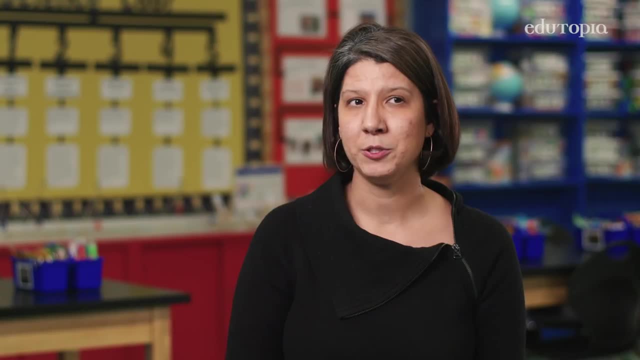 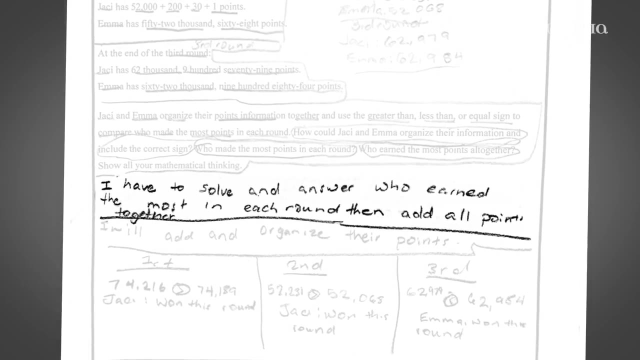 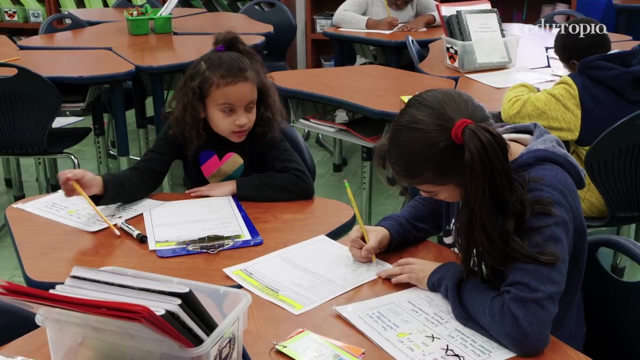 I'm 984.. We also want them to write their I have to statement. What do they have to do in order to solve this problem? It solidifies in their head what the intention and what the goal is of their problem. I think it means how they compare their information. 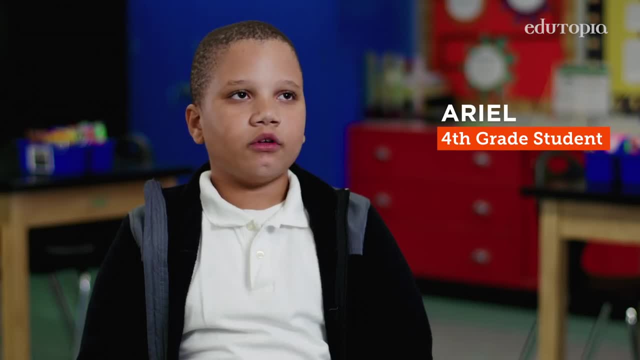 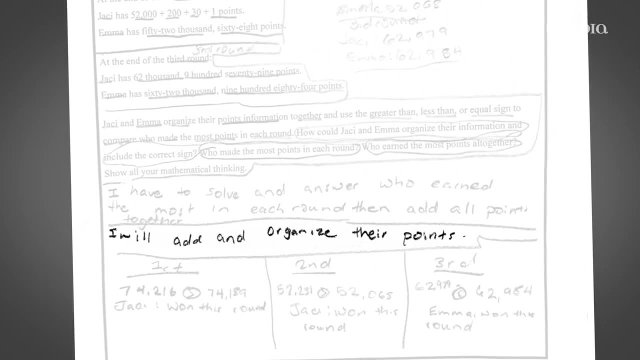 After you understand your thing, you got to think about your strategy and then you do an I will. I will use a table, I will multiply, I will add, I will divide, I will add In the third step they're solving. 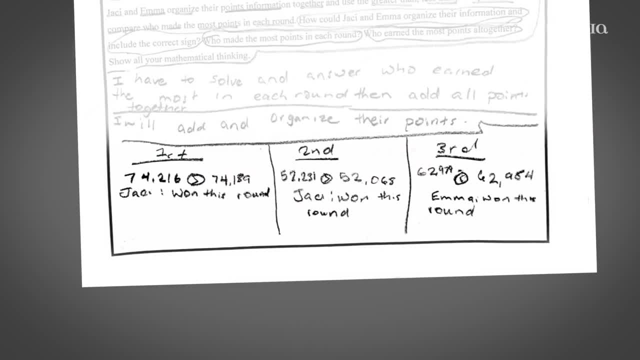 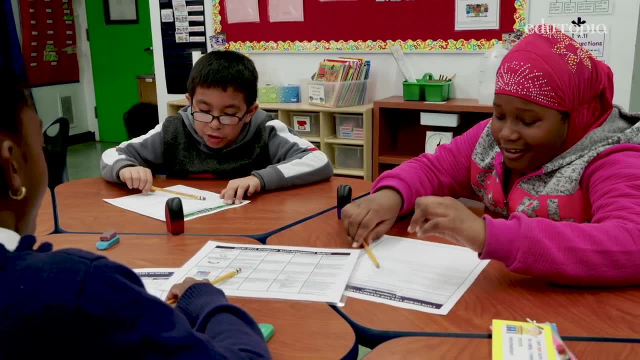 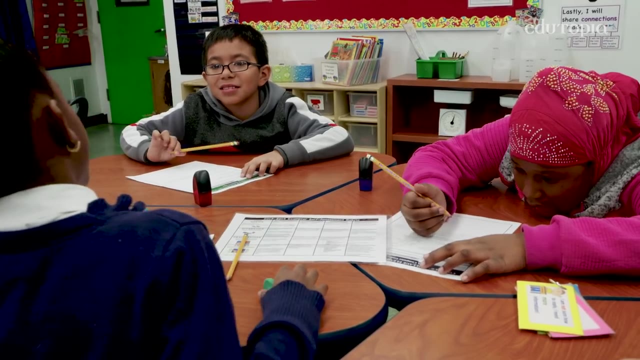 I compared who got the most points in each round and who got the most points all together. I mostly worked by myself and some of the help was from my friends. Look, Rachel, it's 7,000 plus 4,000,. you know, it's 52,000 plus 200.. 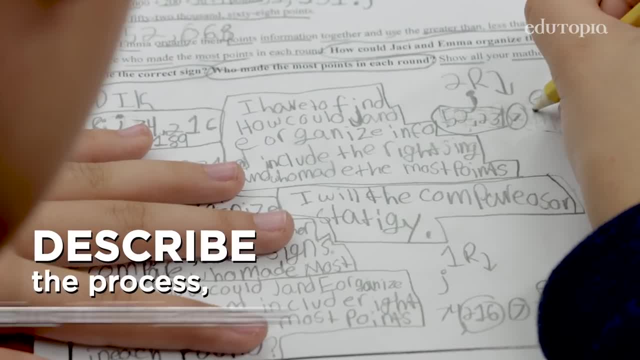 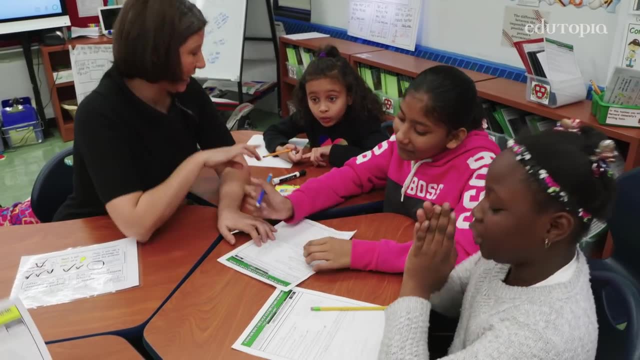 In the fourth step, they are communicating. Their communication involves labeling and making sure that their answers are clearly written and they're explained. When someone looks at your problem- and it's not just you looking at it- they have to understand what you're writing. 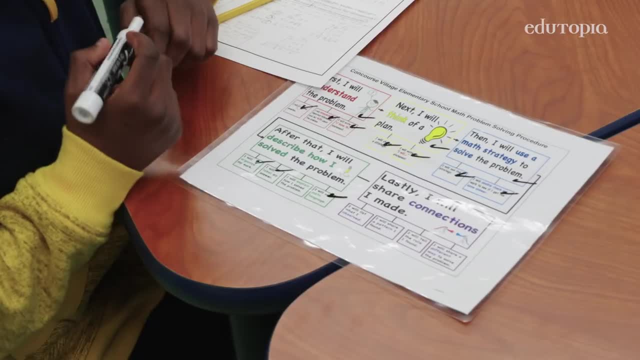 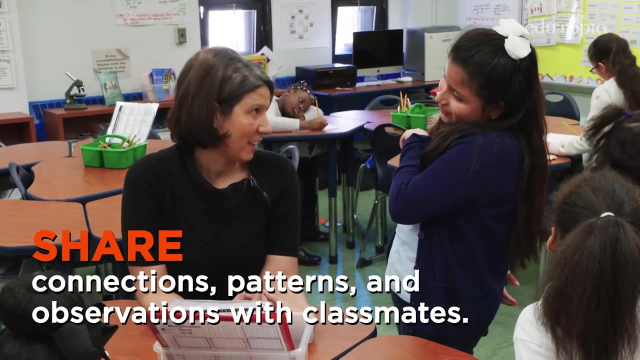 You're trying to show how you're solving the problem. They're going to then create connections regarding any other math that they've done previously. So they're going to look at the numbers, identify if they're even or odd, greater than less.